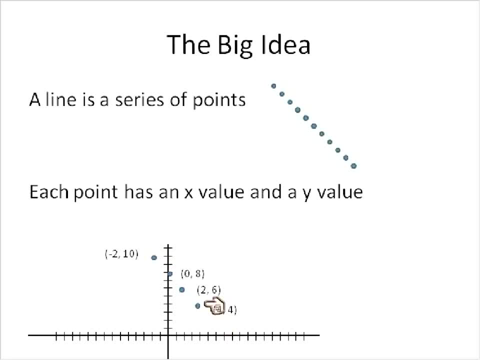 at a line. we're going to be looking at a line. So when we're looking at a line, we're going to have a line and you're looking for the intercepts, you're going to look for the point value or the X and the Y coordinate that corresponds with the point where that 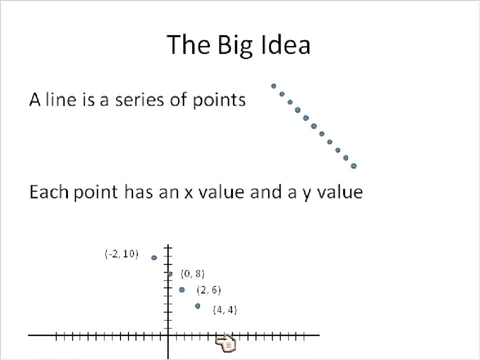 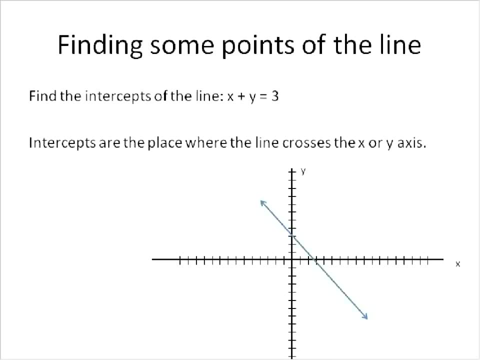 line actually crosses over the X axis, which is this guy, or the Y axis, and that's that one. So here are two major points that we want to find. when we have a line, We want to find the point where it crosses, like I said, the X axis and the Y axis, And this 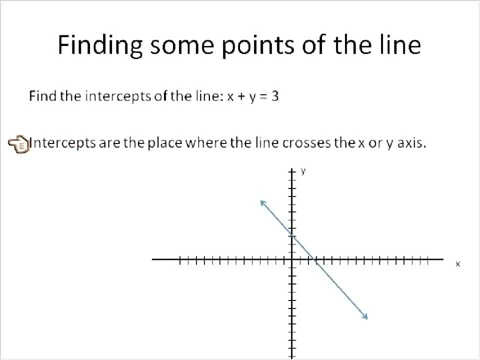 is called the intercepts or the X and the Y intercept. In this case we can look at the graph and we can go: oh well, it crosses the Y axis right about there. So we go 0 on the X axis and we go up 1,, 2,, 3.. 0, 3 is the point where it crosses the Y axis. So 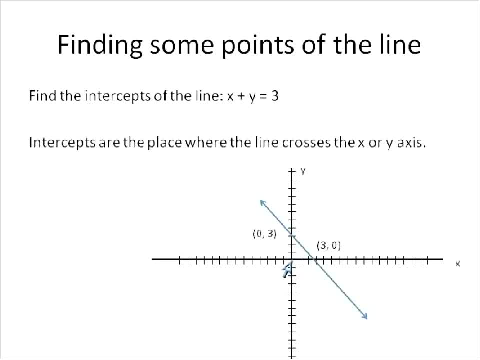 the Y intercept, 0,, 3.. And the X intercept is 1,, 2,, 3, and it doesn't go up. So we're going to go up and down at all. So it's 3, 0.. Well, that's pretty easy when we've got. 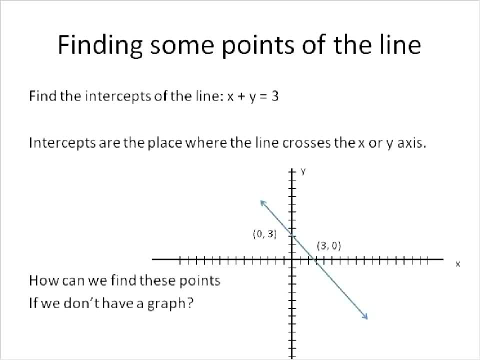 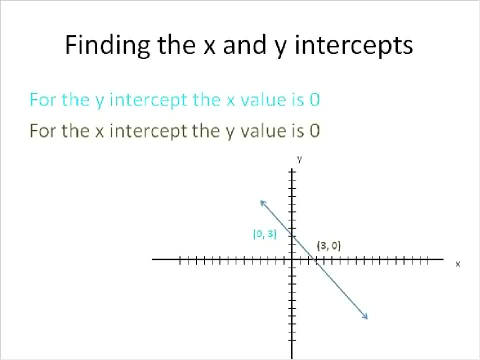 a graph, But how do we find these points when we don't have a graph? That's what we're going to look at today. So the first part that we need to look at here, when we're going to be finding them without a graph, is that we need to notice something For all Y intercept values. 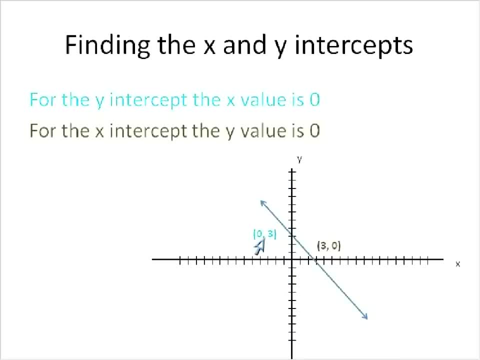 for every single time it crosses the Y intercept, the X axis is going to be the point where the X value will be 0. If we move along the X axis then it's not crossing the Y. For all Y intercept values, the X is equal to 0. We see that here Where it crosses the 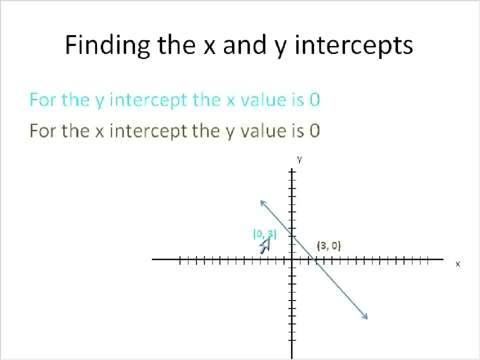 Y axis, the Y intercept, the value is 0, 3.. So for every single time, every time it crosses the Y axis, the X value will be 0.. And every single time it crosses the X value, the X, x-axis, the y-value will be equal to zero. You see that right here. This is the point. 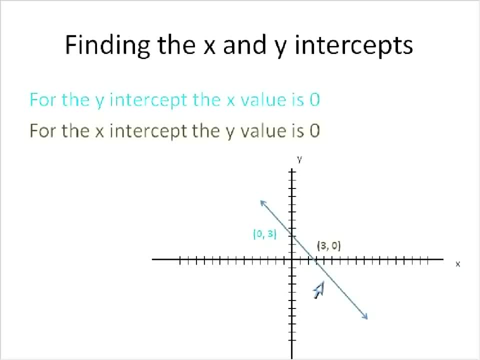 3, 0.. It crosses the x-axis, so the y-value is equal to zero. All right, So that's what we're going to use. We're going to use that information to help us find these points where they actually cross the axis. So we have this equation: x plus y is equal to 3.. If we're 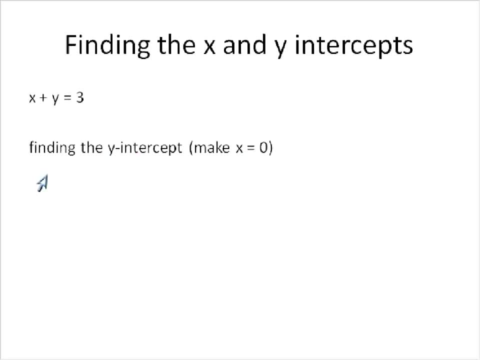 going to find the y intercept, we need to make x equal to zero. So let's take this equation and we're going to plug in zero for the value of x. Look what happens: Zero plus y is equal to 3.. In other words, y is equal to 3.. So our point: if x is 0 and y is 3, our point is: 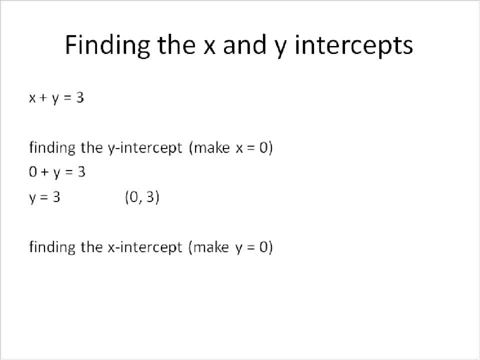 zero, 3.. Let's find the x-intercept. For the x-intercept we're going to the x-intercept, we're going to make y equal to 0.. So to do that, we get our original equation and we plug the value. 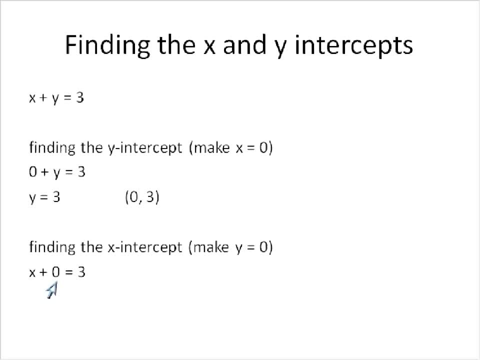 of 0 in for y. x plus 0 equals 3.. Well, if x plus 0 equals 3, then x is equal to 3.. x is equal to 3,, y is equal to 0.. We've just found our point: 0,, 3, and 3, 0.. Mathematically, 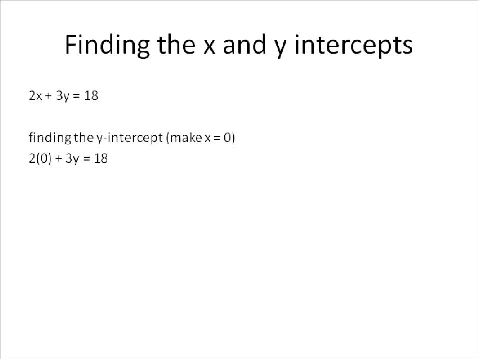 instead of using the graph that we had, Let's look at another question, a little bit more complicated this time We have the equation: 2x plus 3y is equal to 18.. That's our equation. If we want to find the y-intercept, we need to make x equal 0.. So everywhere we see an. 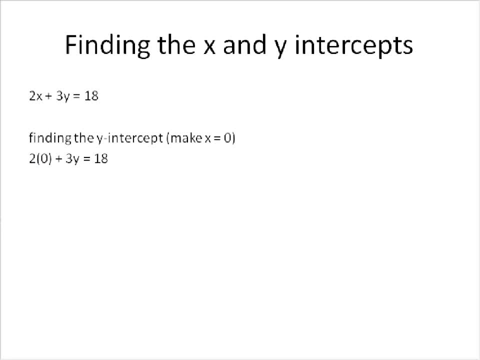 x, we're going to plug in a 0.. 2 times 0 is 0,, so the 2 essentially removes itself. And then we divide both sides of this equation by 3, and find that y is equal to 6.. So when 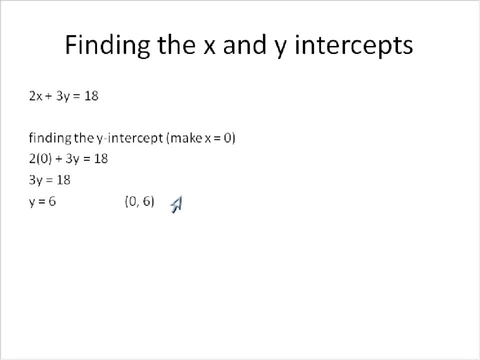 x is equal to 0, y is equal to 6.. That is our y-intercept. All right To find the x-intercept. we make y equal to 0. So we're going to plug 0 into this equation, and that's just from. 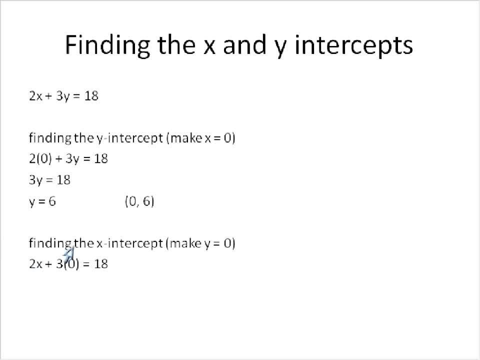 the original equation. we have 2 times x, 3 times 0. And 3 times 0 removes itself right. It is equal to 0. So now we need to find the value for x. We divide both sides by 2 using the property of equality, And we have x is equal. 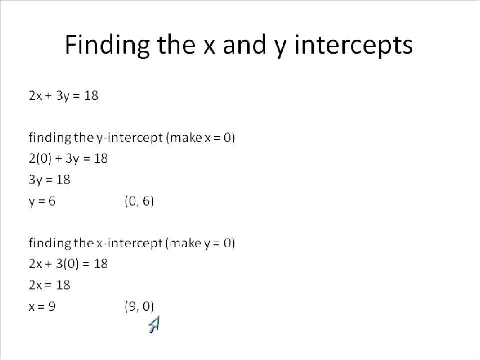 to 9.. x is equal to 9 when y is equal to 0.. That is our x-intercept point. All right, I'm going to do one more example. And this type of question, it really requires some practice. So, doing it over and over and over, you'll start to see patterns. You'll start. 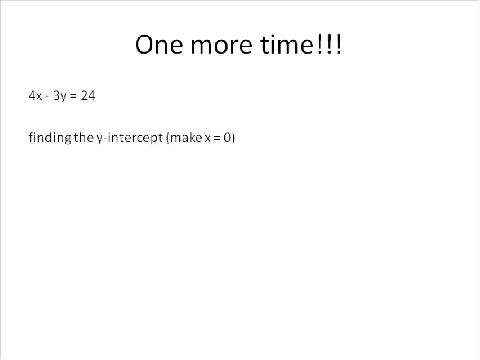 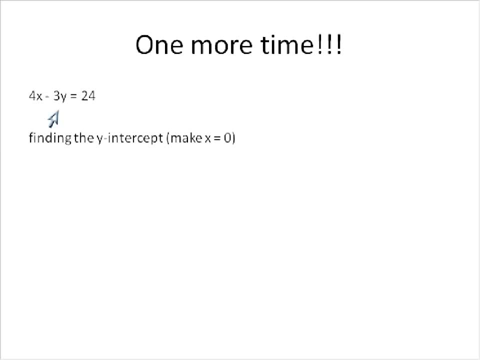 this one again a third time here a different equation: 4x minus 3y equals 24.. We're going to find the y-intercept. To do that we need to make x equal to 0.. 4 times x or 4 times. 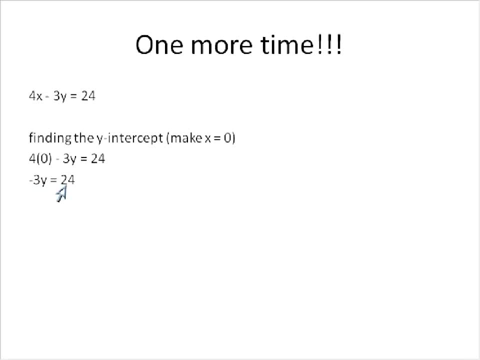 0 is equal to 0. So essentially we're looking for negative. 3 is equal to 24.. We divide both sides by negative 3. And we find that y is equal to negative 8. So our y-intercept point is 0, negative 8.. 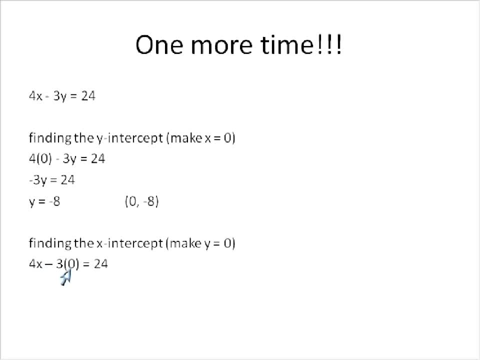 For finding our x-intercept. we make y equal 0.. Plug that 0 into the equation. 3 times 0 is 0.. 4x minus 0 is the same as saying 4x. So now we solve for 4x. We'll divide both. 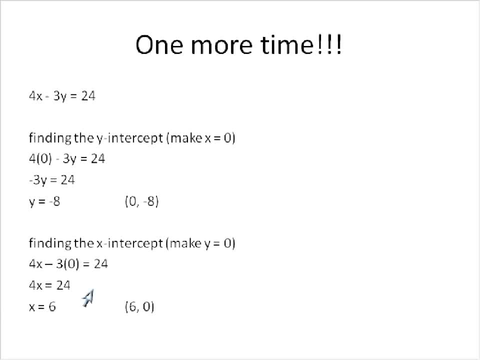 sides of the equation by 4.. 24 divided by 4 is 6.. And 4x divided by 4 will just give us x. So using the property of equality again, we found that x is equal to 6 when y is equal to 0. So that's going. 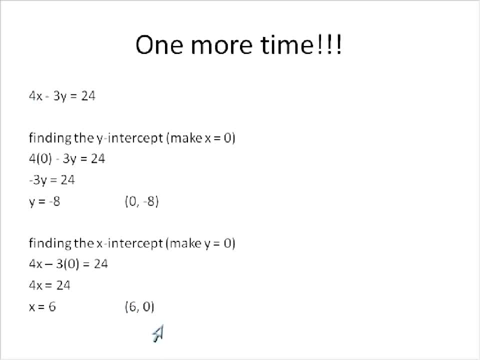 to be a point on this line. Specifically, it's going to be the x-intercept point. So that's the way that you find x and y-intercepts. If you're looking for the y-intercept, make x equal 0 and solve for the y-intercept.